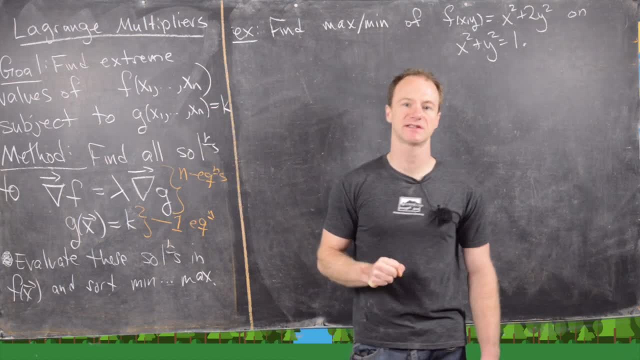 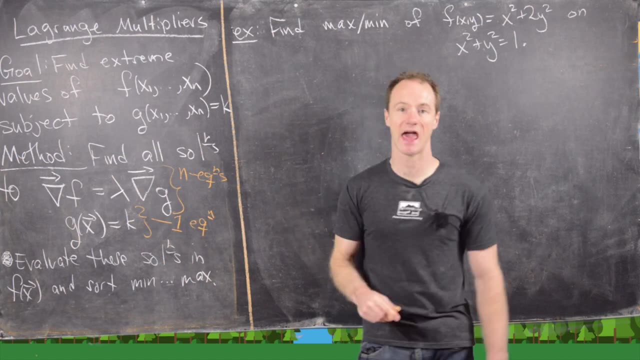 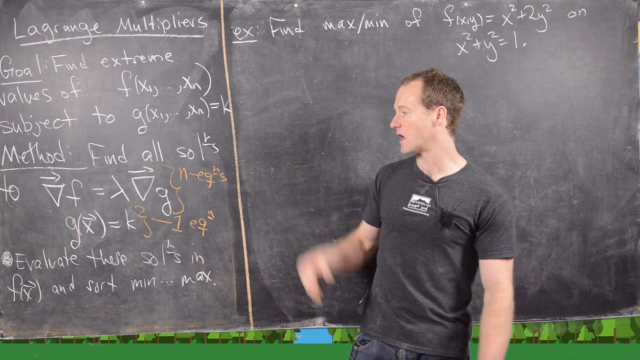 the absolute max and min of this function subject to some constraint equation, And that constraint equation is given by g of x1 to xn equals k. Okay, great. So the method goes in the following way: We want to find all solutions to the following system of equations: 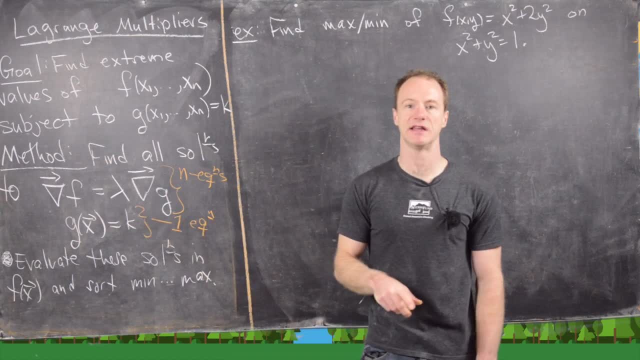 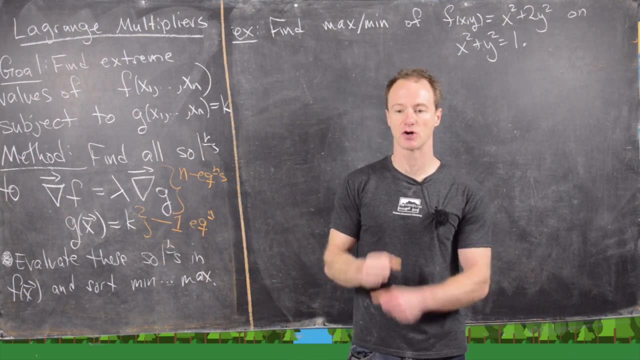 So we have the gradient of f equals lambda times the gradient of g. That's in equations really, because, remember, the gradient is going to be a vector which has as many entries as variables from the original function. So the original function is x1 to xn and we want to find the extreme values of x1 to. 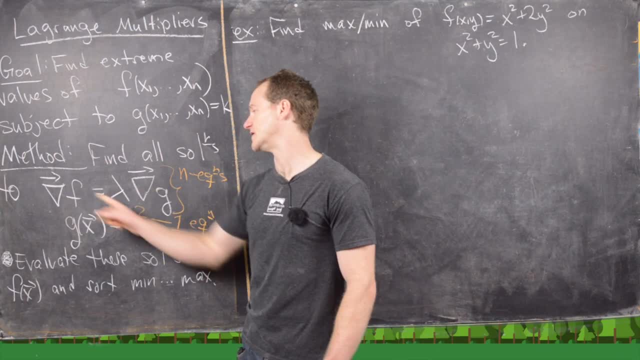 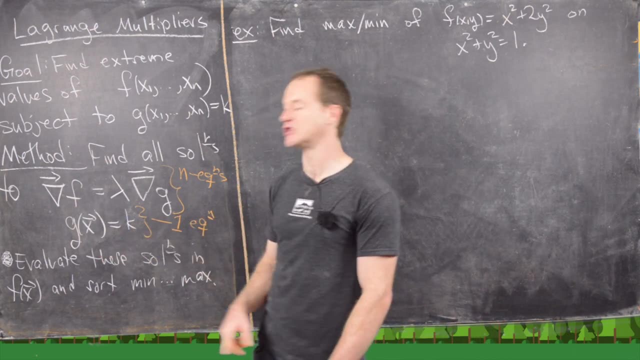 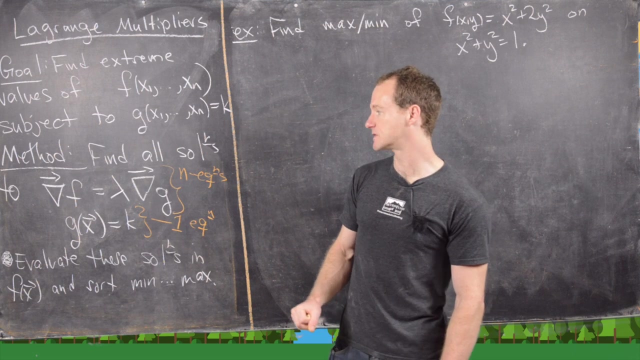 xn. So this is going to be a vector equation with n entry vectors, which means it's n scalar equations. And then we have one more equation, given by the constraint equation. So now notice that is exactly n plus one variables and n plus one unknowns. So our sorry, n plus one. 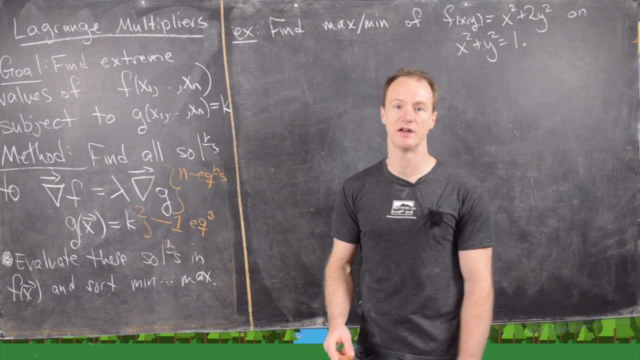 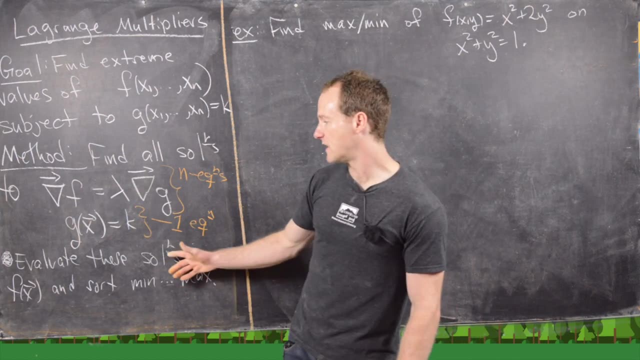 variables and n plus one equations. So we have n plus one equations, and then our unknowns are x1 to xn and this lambda, Okay, great, And then we'll evaluate all of those points. so the x1 to xn points in the original function. 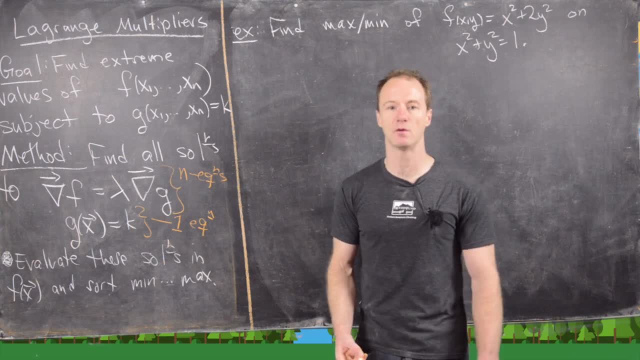 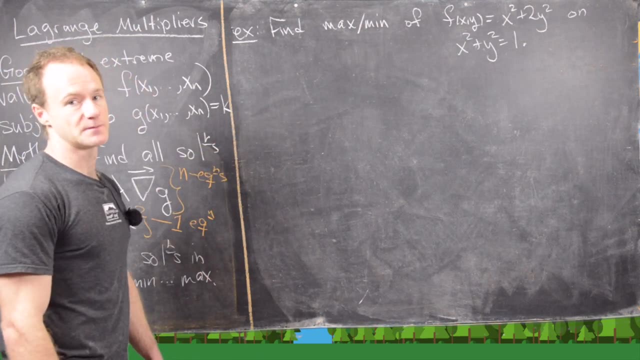 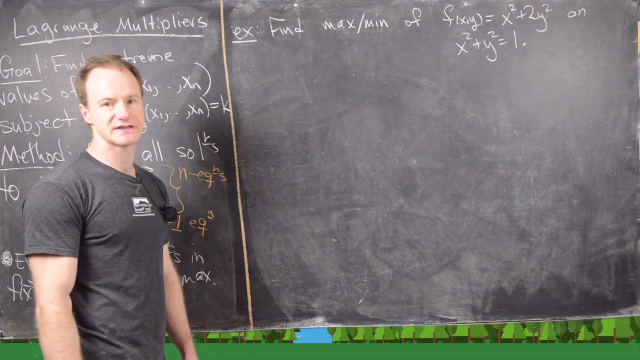 and sort them from minimum to maximum, and then we'll have our absolute maxes and mins. Okay, so let's look at this example. So we want to find the max and min of this function. f of xy equals x squared plus two y squared on the unit circle, So in other words, x squared. 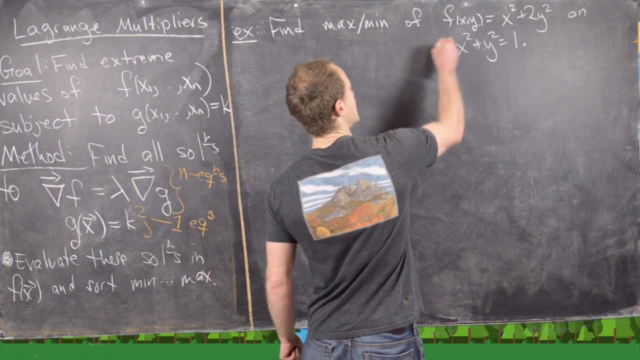 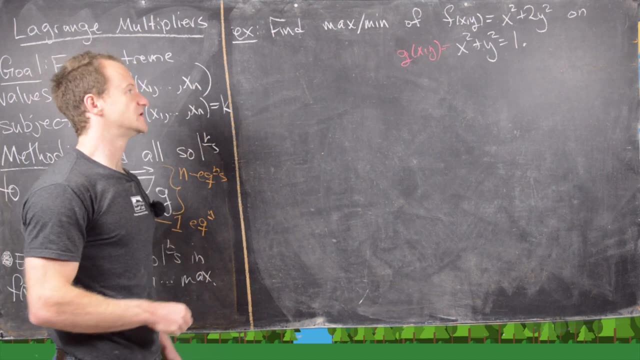 plus y squared is one. So notice this guy right here. He's playing the role of g, of xy in this case, And we also only have two variables, so this should be pretty simple. Okay, so we've got two types of equations we need. We need the. 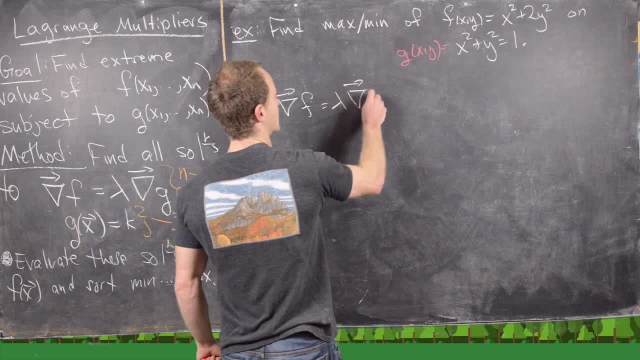 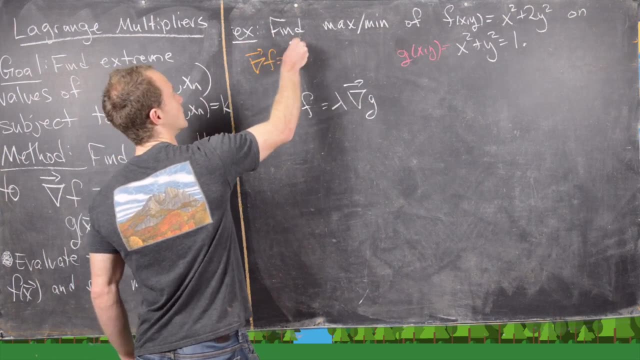 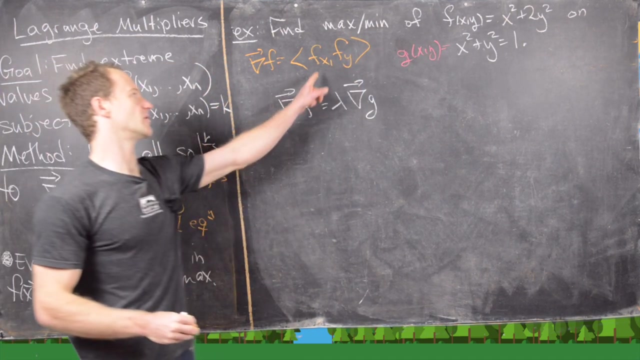 gradient of f to be equal to lambda times the gradient of g. So let's recall real quick that the gradient of f is going to be the vector made up of partial derivatives of f, And if there are n variables, then it'll be the derivative with respect to the first, second, third, and so on and so forth. 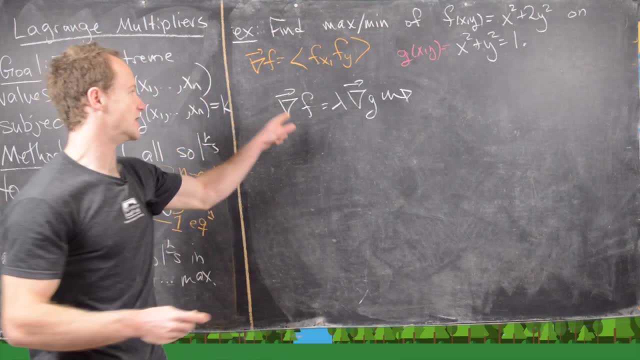 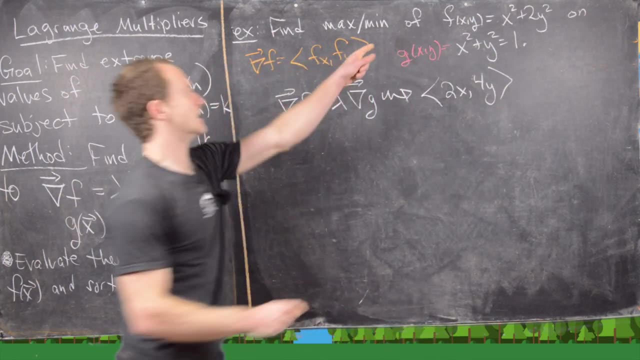 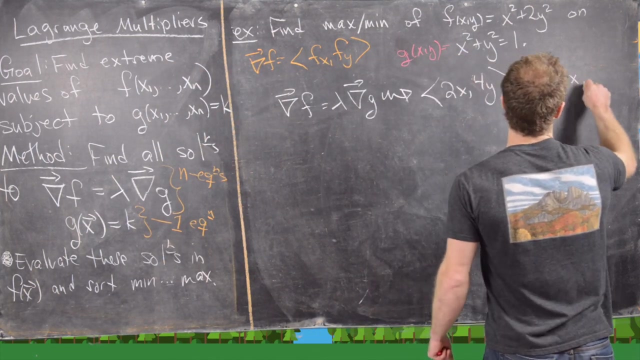 So notice, that's going to give us the following vector equation: So we'll have 2x comma 4y, So that is the gradient of f for our function, And then that needs to be equal to lambda times 2x times 2y, And that is the gradient of our g function. Okay, great. 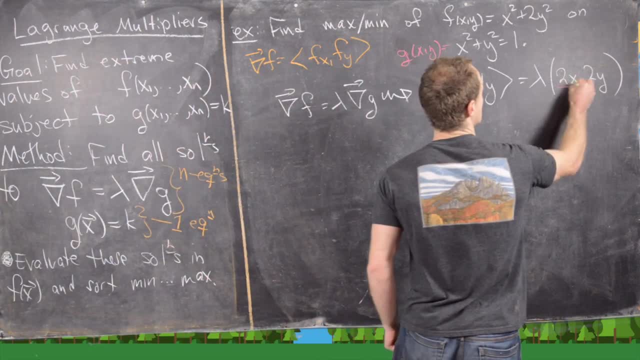 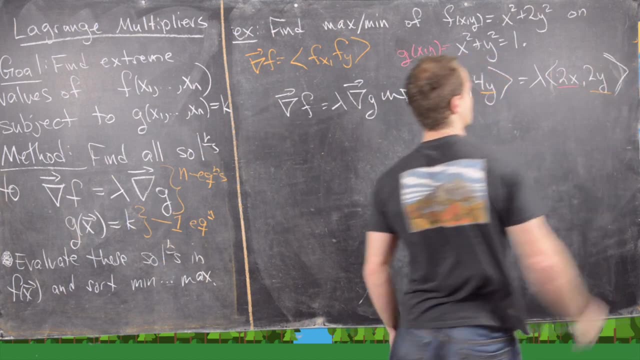 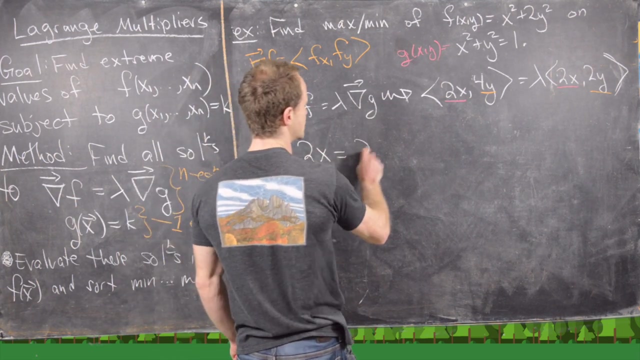 So now notice that we have the gradient of f for our function, And then that is the gradient of f for our function. So notice, we can extract entries from these vectors, keeping in mind that we need to scalar multiply by this lambda, And that will give us our system of equations. So notice, we'll have 2x needs to be equal to 2 lambda x. 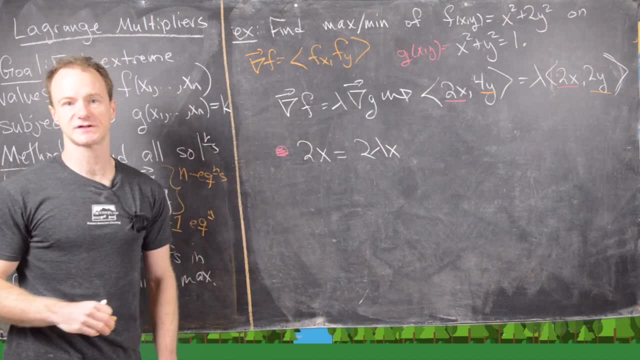 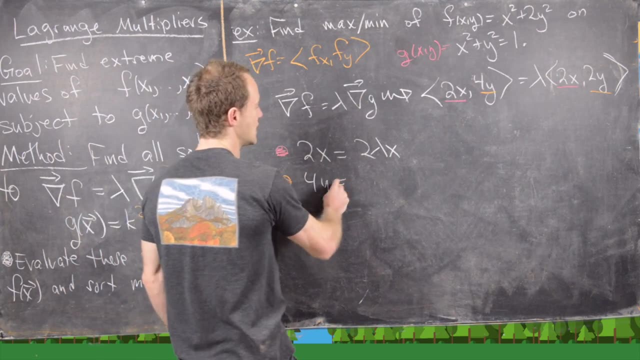 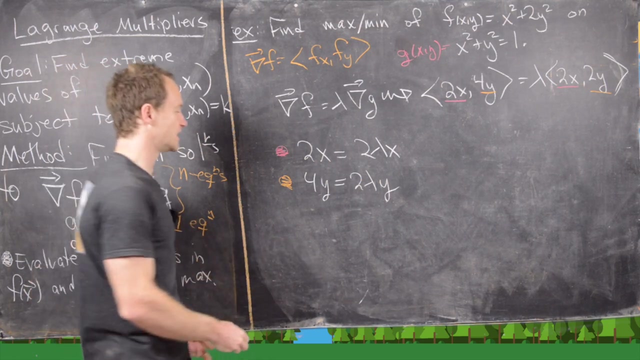 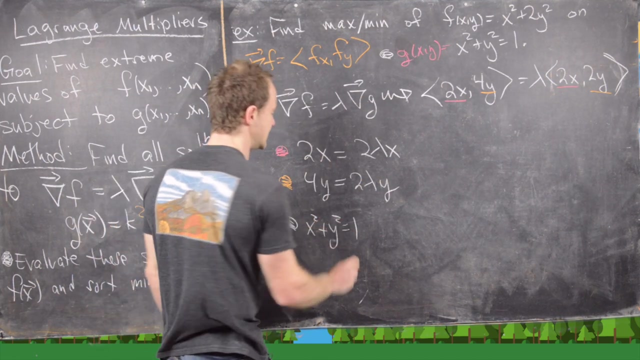 So we get that from extracting from the first entry of our vector. We can extract from the second entry of our vector to get 4y equals 2y And then finally we have our constraint equation which is like given, And that is: x squared plus y squared needs to be equal to 1.. 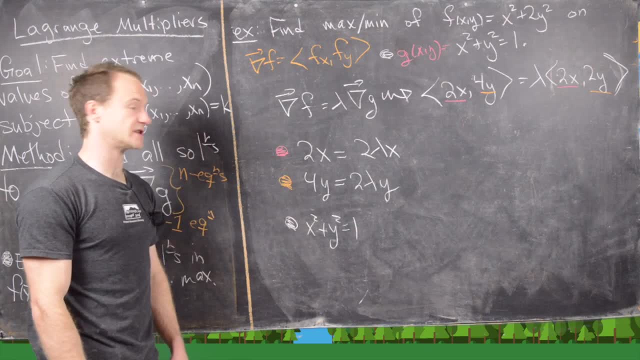 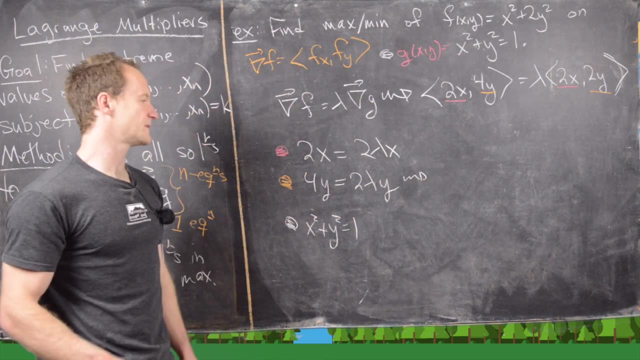 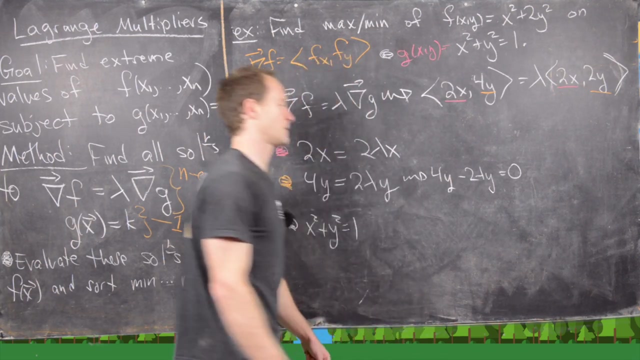 Okay, good, So now let's see if we can solve this system of equations. Okay, so let's go ahead and start with this one So we can move some things around and notice we will get 4y minus 2 lambda y equals 0.. 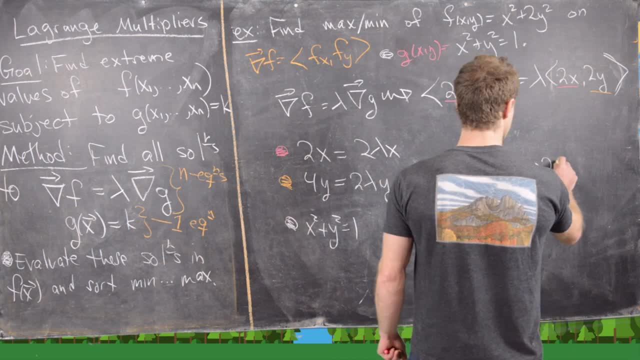 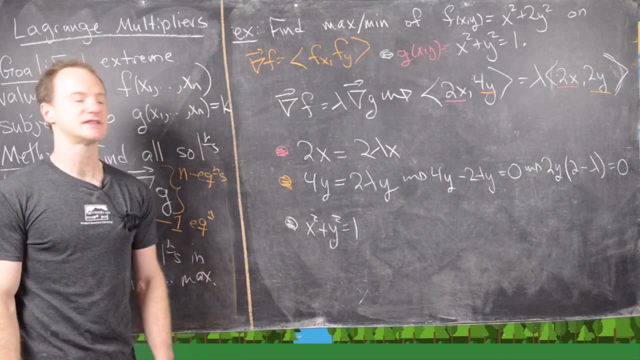 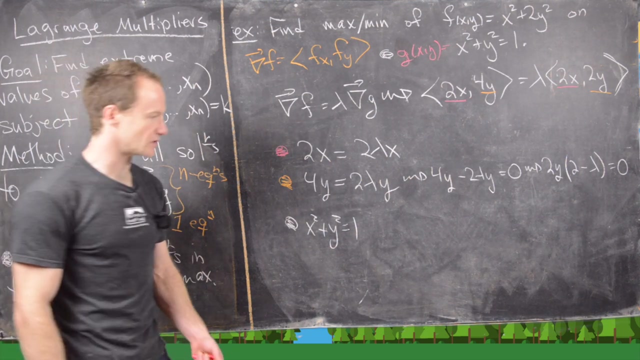 And now we can factor some things about who we got this, And I notice that's going to give us 2 times y, And then we'll have 2 minus lambda equals 0.. So we've got 2 cases to work with. Either y is equal to lambda- sorry, y is equal to 0 or lambda is equal to 2.. 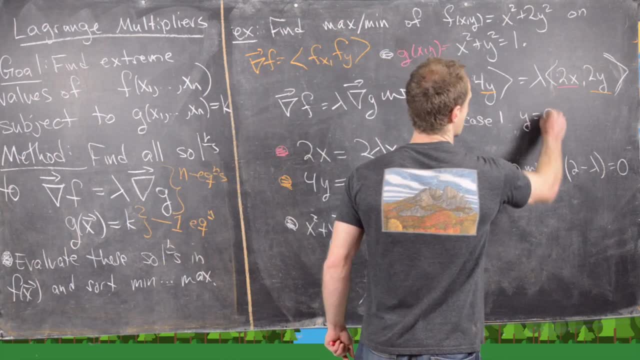 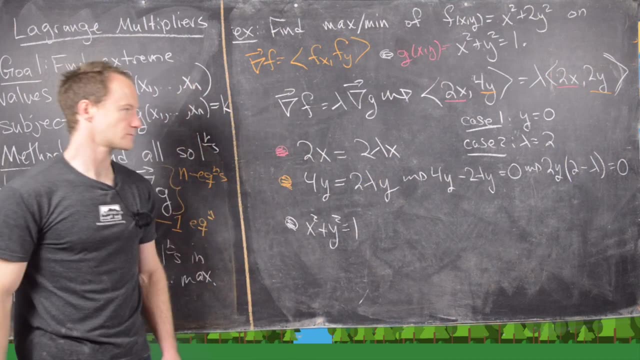 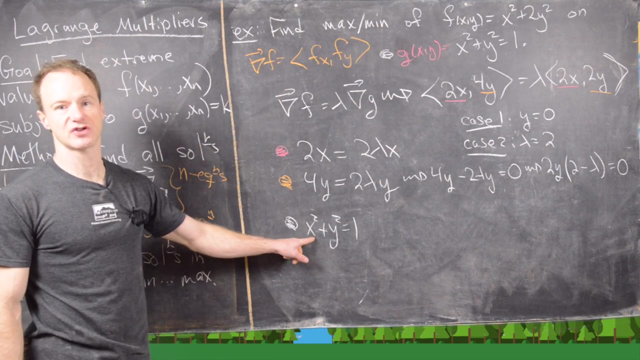 So let's all write that down. So case number 1 would be y equals 0.. Case number 2 is y equals 0.. 2 would be lambda equals 2.. But now let's go ahead and plug in y equals 0 into this constraint. 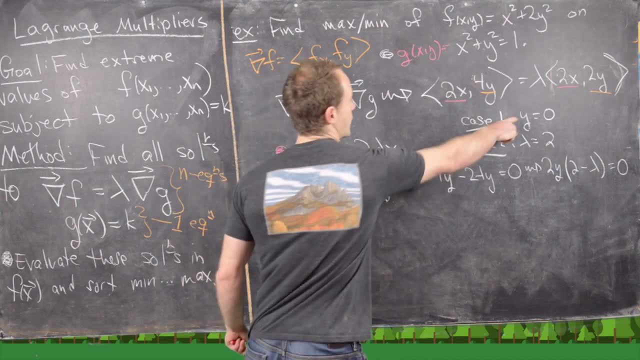 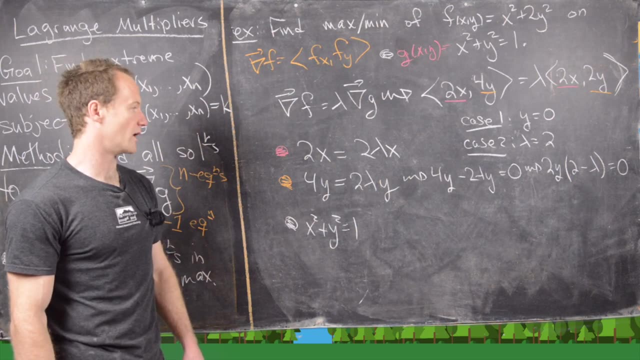 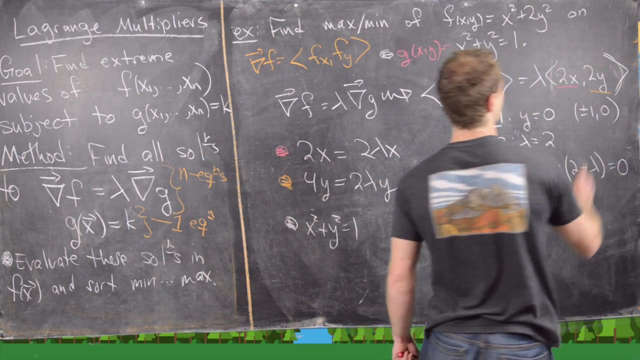 equation down here, And so notice, if y equals 0 gets plugged into this constraint equation down here, we get x equals plus or minus 1.. So let's see, that will give us the points plus minus 1 comma 0.. Okay, great, And now the next thing that we want to look at is what happens if 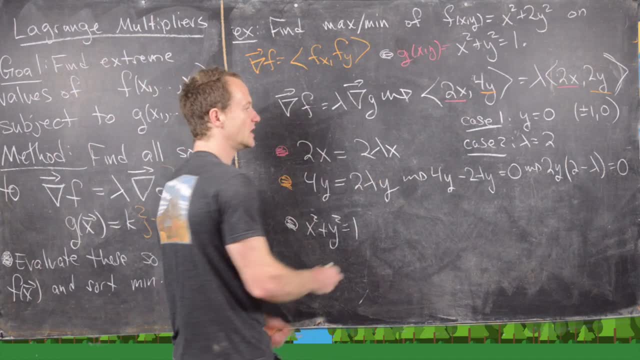 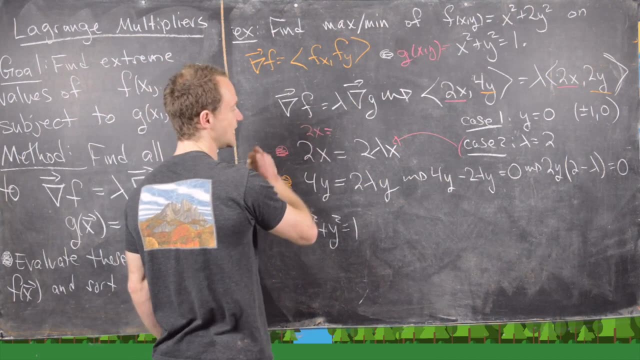 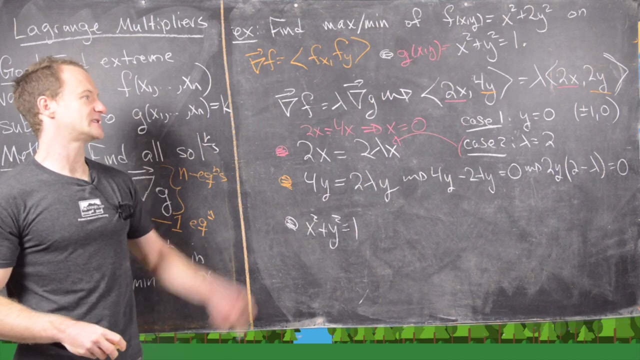 lambda equals 2.. So if lambda equals 2 gets plugged into this equation, that will give us 2x equals 4x, which tells us that x has to be equal to 0. So that means case 2 will give us: 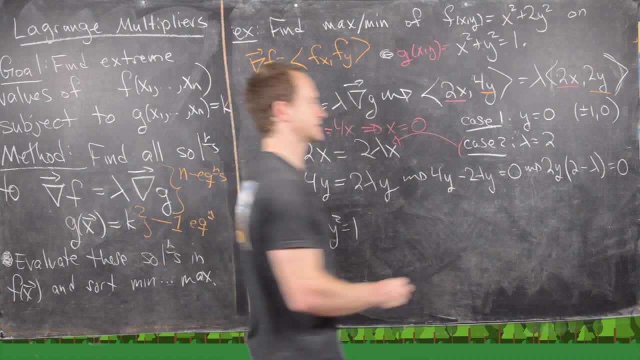 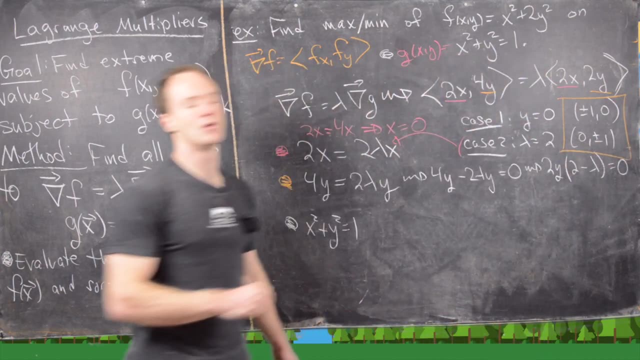 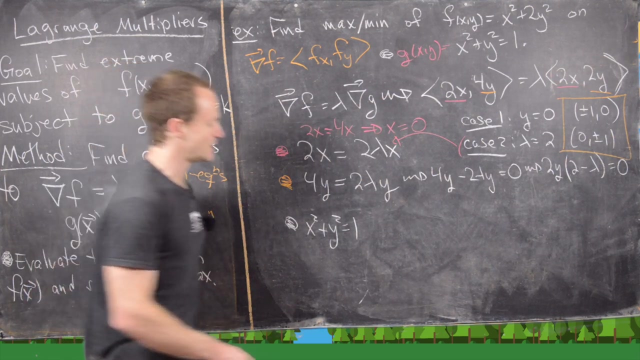 x equals 0, which means y has to be plus or minus 1.. So we have 0 plus minus 1.. So by solving the system of equations we have found that these four points are the important points for this setup. So that means we can take our points. 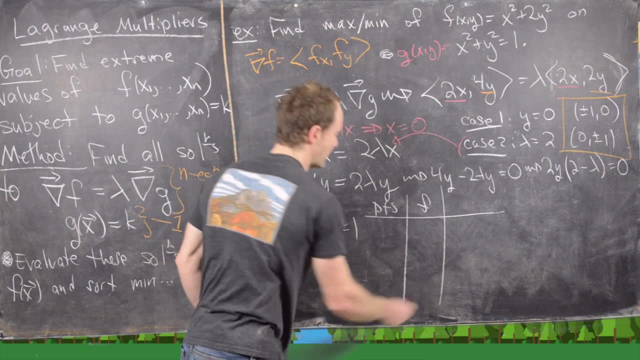 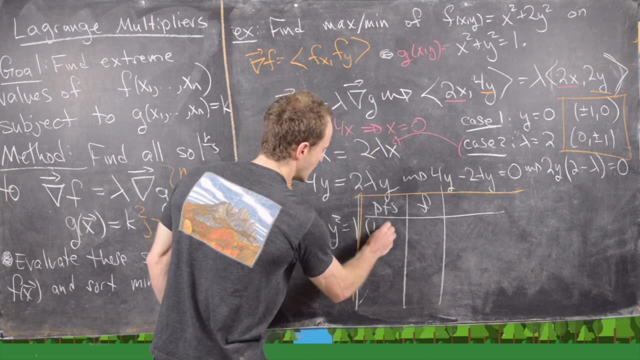 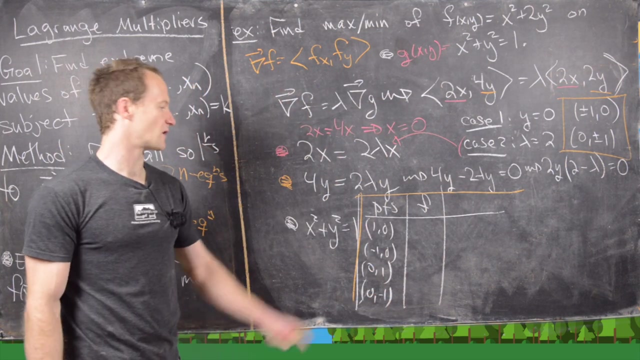 and our function and then evaluate them. So let's see we've got our point: 1, 0 minus 1, 0.. 0, 1, and 0 minus 1.. So let's plug those into our function, So 1, 0 into our original function up. 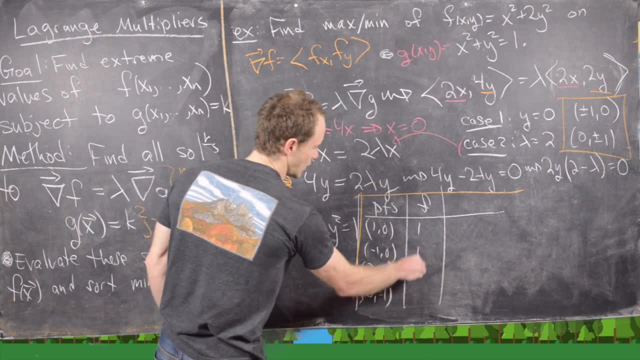 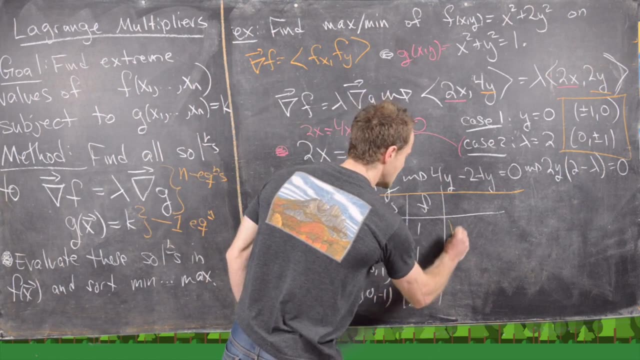 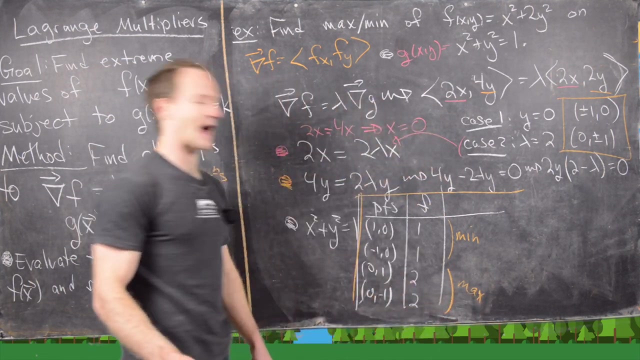 here will give us 1.. Negative 1, 0 will also give us 1.. This will give us 2, and this will also give us 2.. So notice, we have a minimum at those two points and we'll have a maximum at the last two. 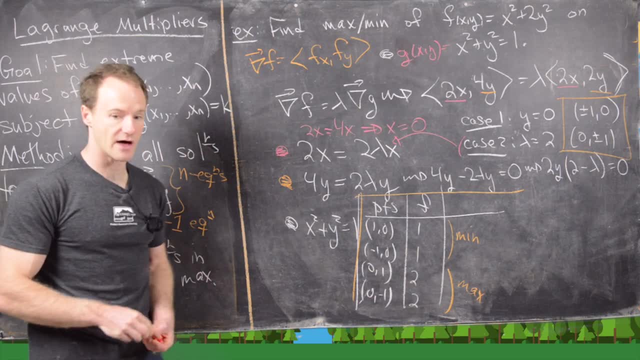 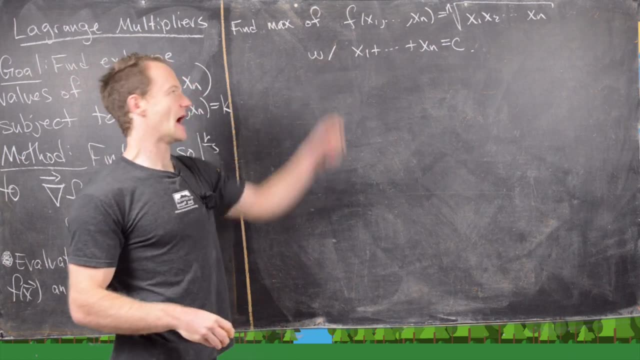 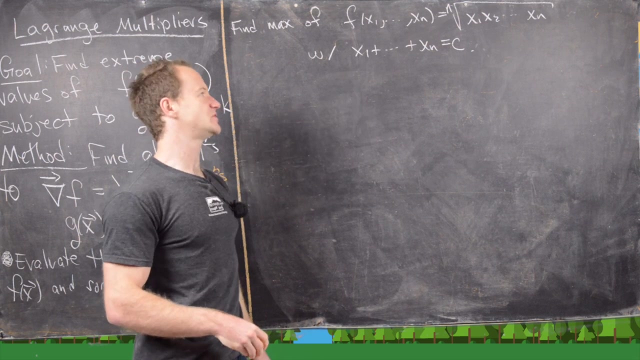 points. Okay, I'm going to clean up the board and then we'll do a little bit of work on the next example. Okay, so for our next example, we want to find the maximum of this function given by f, of x1 to xn. is the nth root of this product, x1 to xn, and it's going to be subject to this. 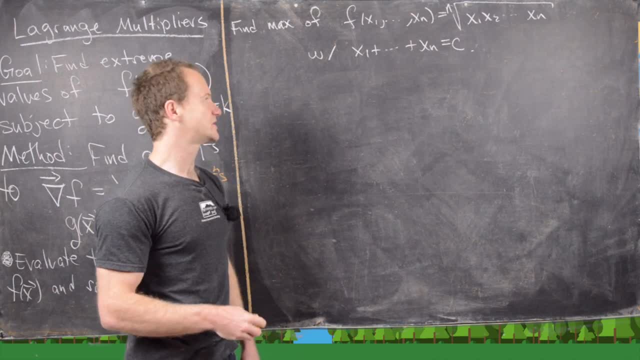 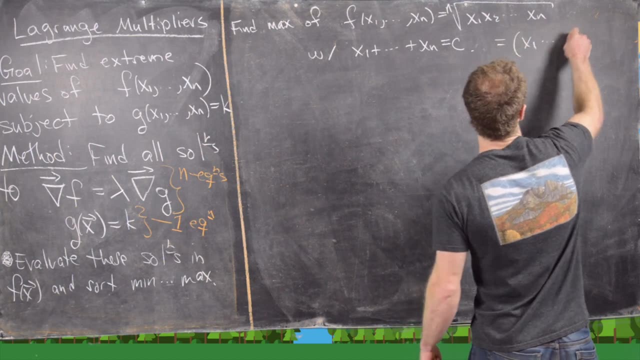 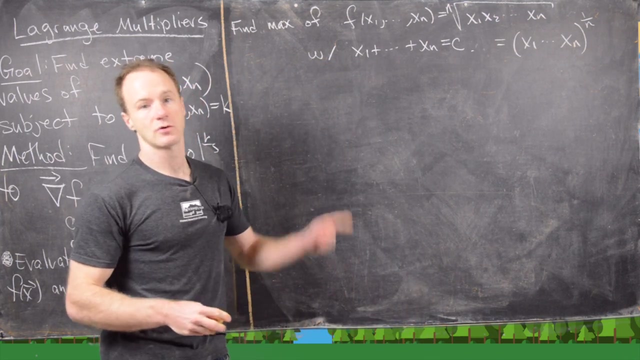 constraint that x1 plus x2 all the way up to xn is a constant c. And here maybe, first I want to notice that this is the same thing as x1 times up to xn, to the 1 over n Power- Okay, great. And then maybe also notice that that is going to give us x1 to the 1 over n. 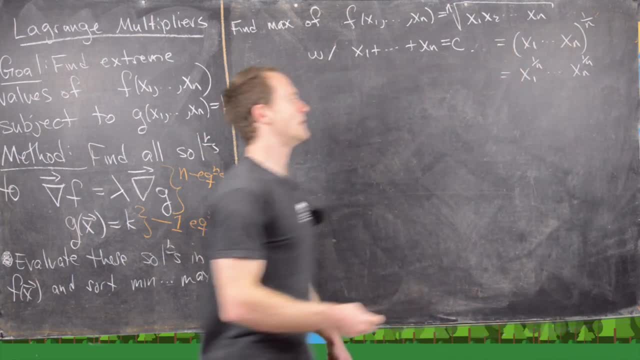 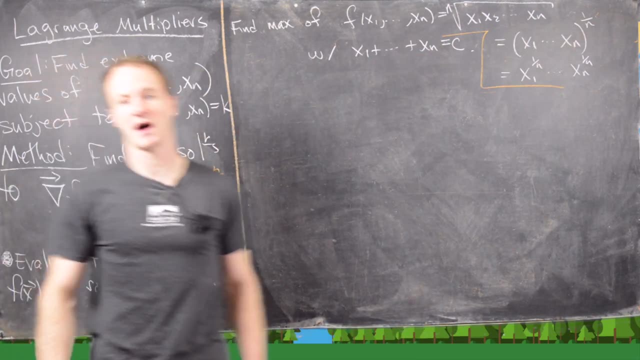 all the way up to xn, to the 1 over n, So maybe that'll be a helpful way to think of it in a bit. Okay, great, Now notice for the method of Lagrange multipliers. we need to find the gradient of these. 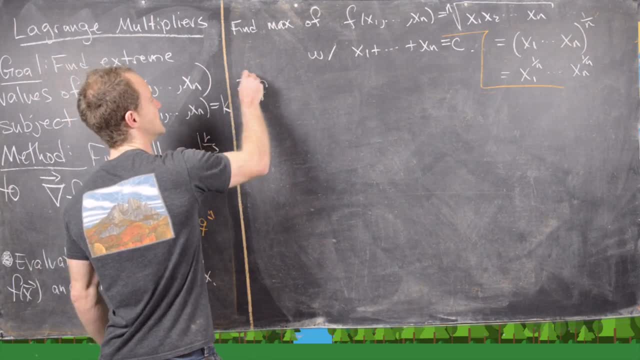 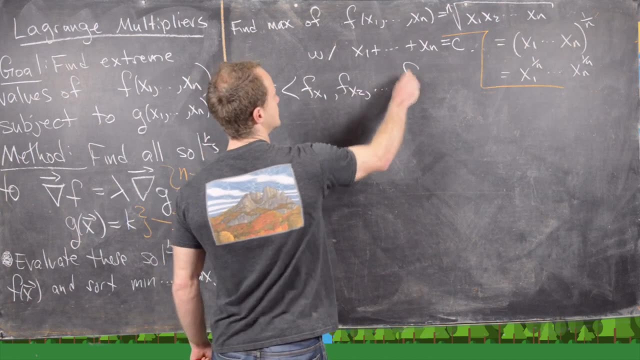 two functions. So let's just recall that in this invariable case, the gradient of f will be the partial with respect to the gradient of f. So we're going to find the gradient of f and we're going to have the partial with respect to x1, the partial with respect to x2, all the way up to the. 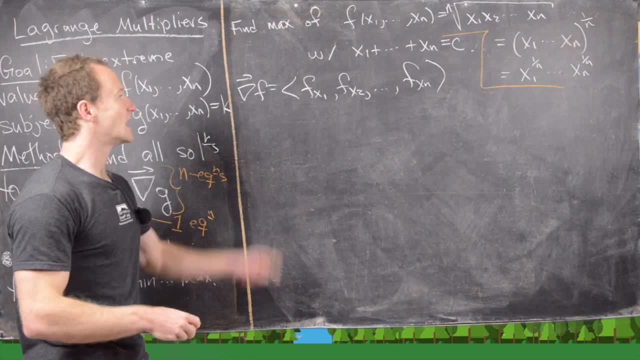 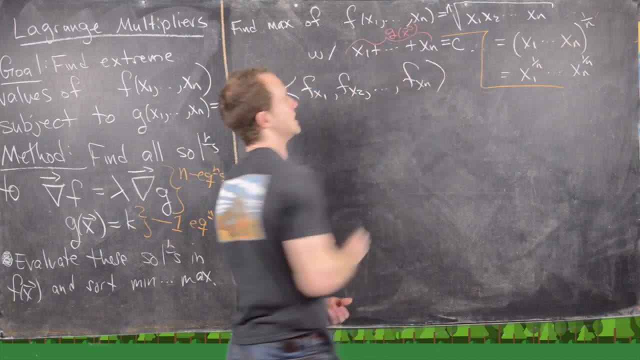 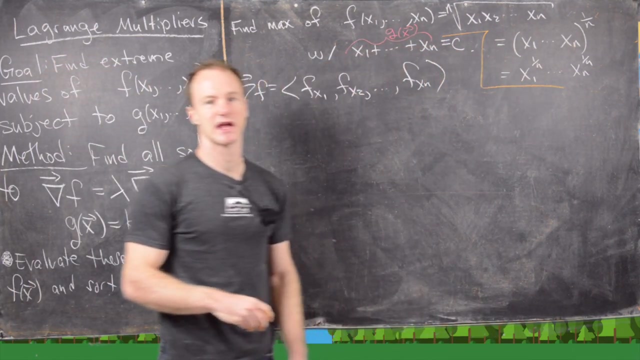 partial with respect to xn, So that will be an n vector, And then we'll have something similar for g, and the role of g is being played by this function right here in this case. Okay, good. So now also, let's notice that f is symmetric in all of these variables, In other words, 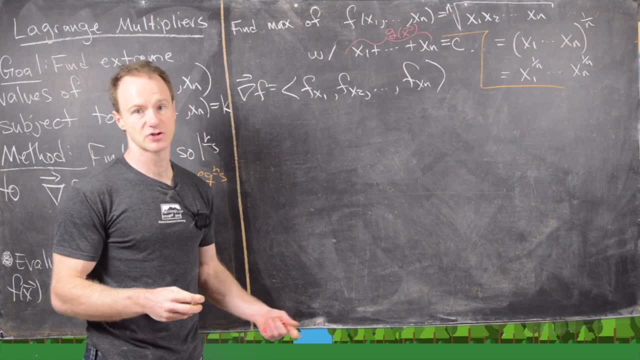 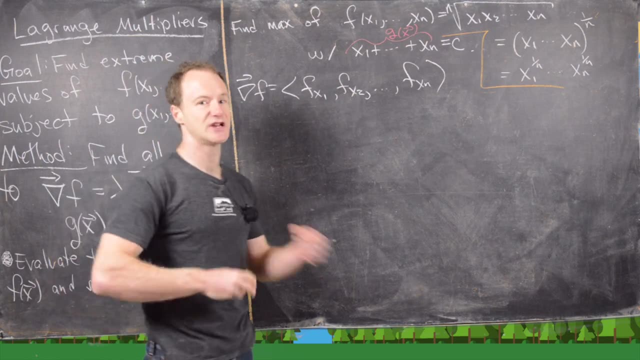 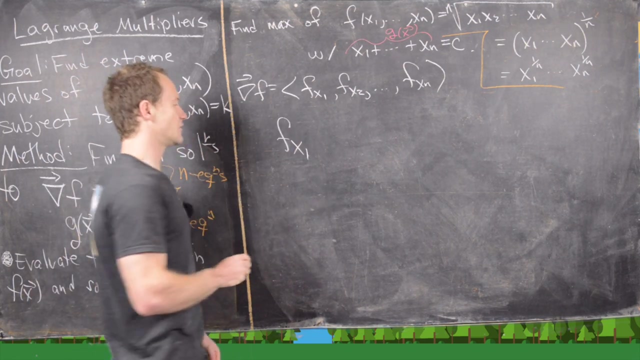 if we rearrange these variables, we get the same function. So what that means is, if I take the derivative with respect to x1 or the derivative with respect to x2, we should get a similar result that just replaces x1 with x2.. So I'm going to go ahead and take the derivative. 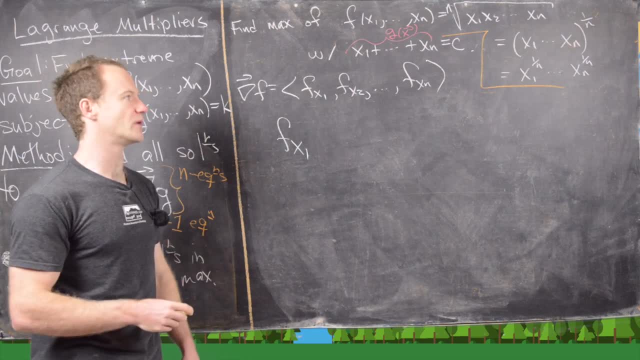 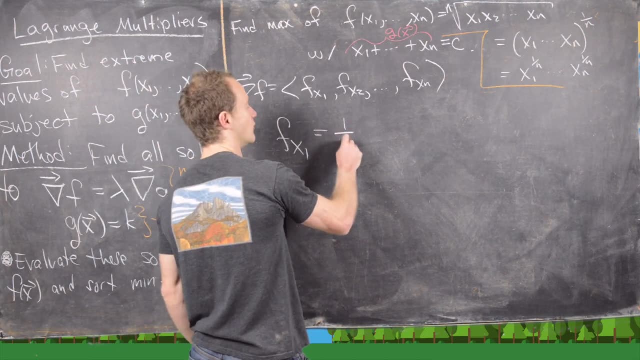 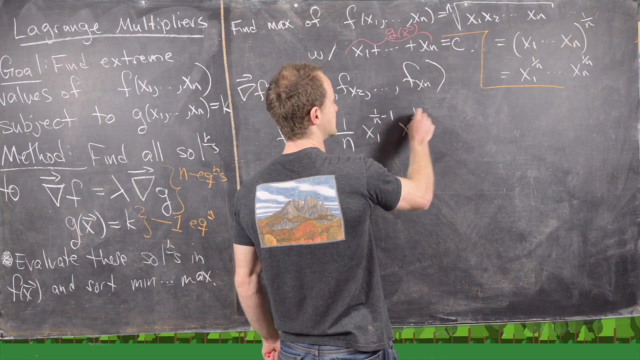 with respect to x1, and then that will allow us to argue what the derivative is with respect to everything else. So notice: the derivative with respect to x1 will be the following: We'll have 1 over n times x1 to the, 1 over n minus 1 times x2 to the. 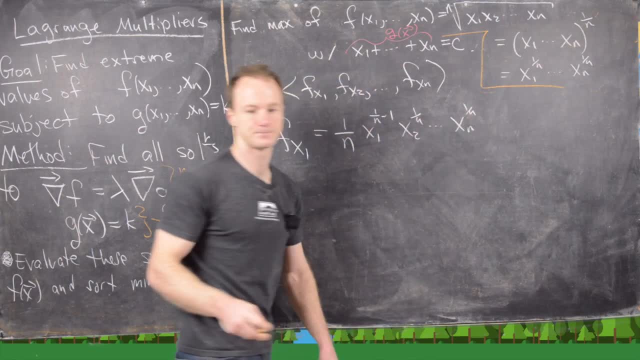 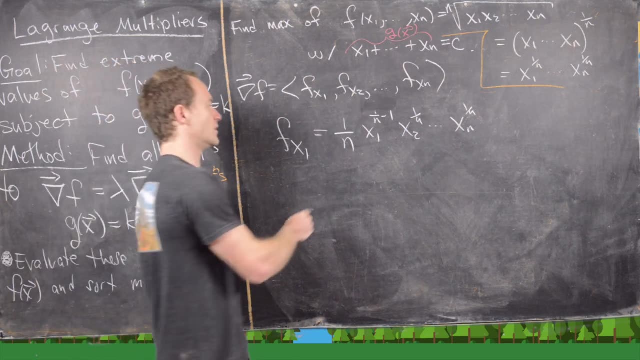 1 over n all the way up to xn to the 1 over n. Okay, so we've got something like that. Okay, so now the next thing that we want to notice is that we can rewrite this as x1 to the 1 over n. 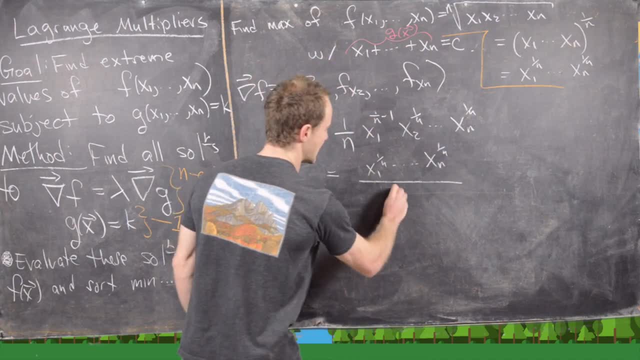 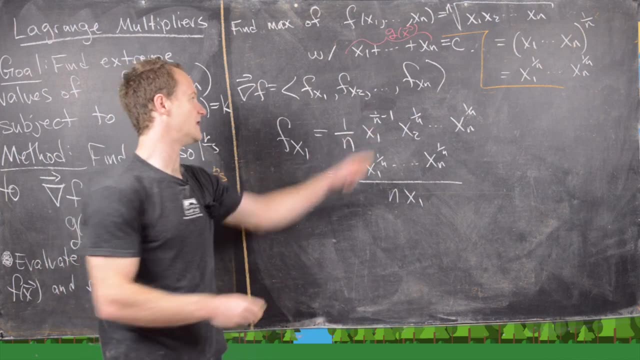 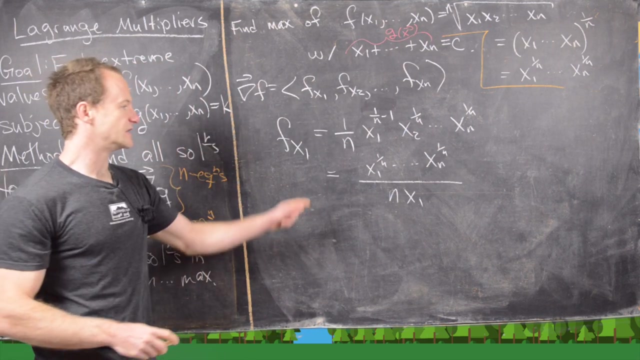 times up to xn to the 1 over n. all over n times x1.. Okay, so notice this: 1 over n. I just made an n in the denominator and then, instead of having 1 over n minus, I just put an x1 to the first power in the denominator, and so this is equal to. 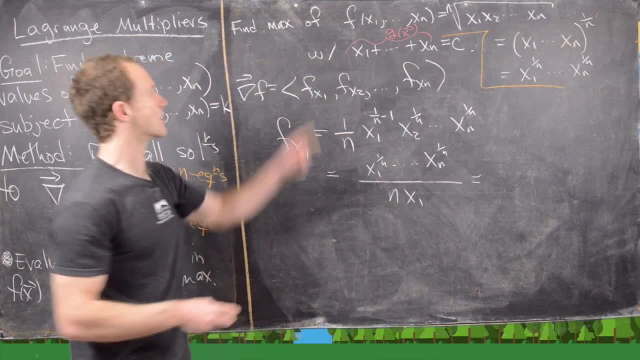 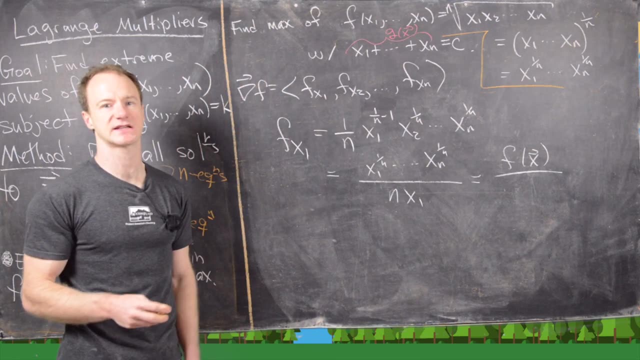 Okay, so now notice that we can rewrite this numerator as the original function, So I'll just go ahead and write that as f applied to the vector x, where by vector x I mean x1 to xn, and now I have n times x1 in the denominator, and then now similarly. 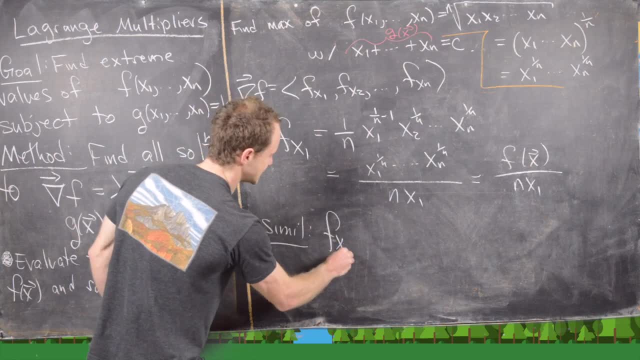 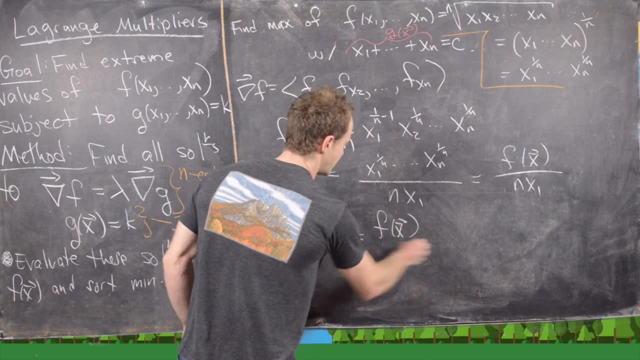 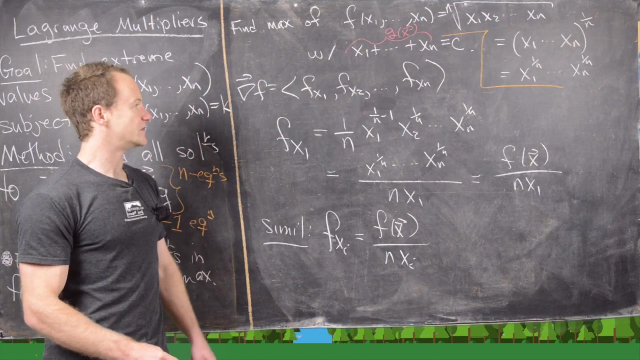 We'll have the same equation for all of these derivatives. with respect to x i, this will be equal to the original function divided by n times that variable x i. Okay, good, So now i'm going to clean up this part of the board and then we'll use that. 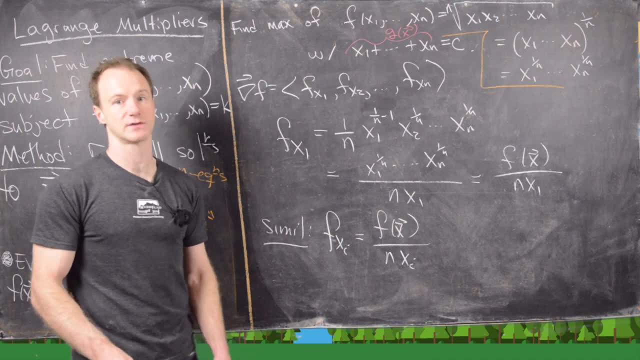 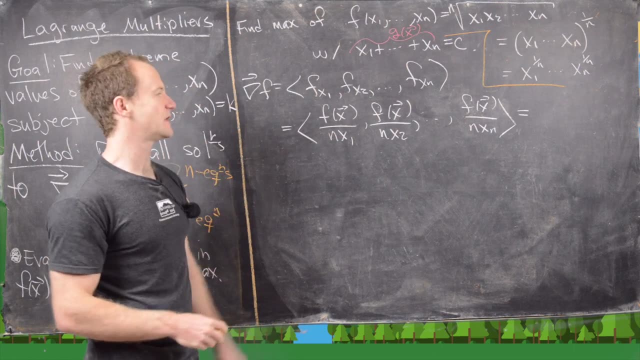 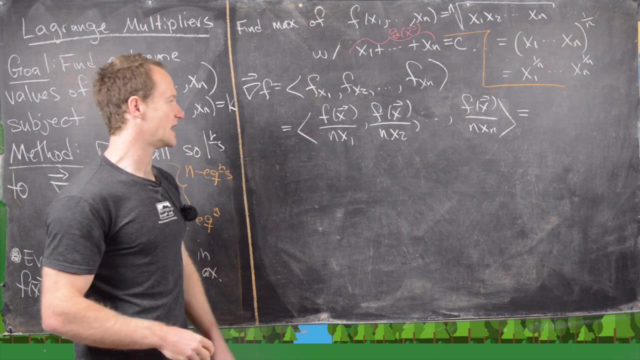 To write down a formula for the gradient. That's really nice. Okay, so in the previous board we calculated all of these partial derivatives of our function f, so now I put them together into this gradient vector. so I have function f divided by nx1, function f divided by nx2 all the way up to function f divided by nxn, and 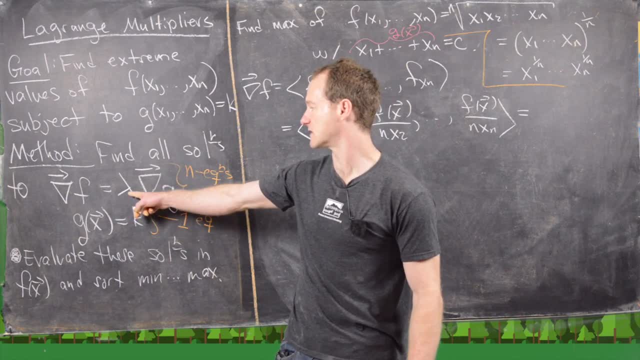 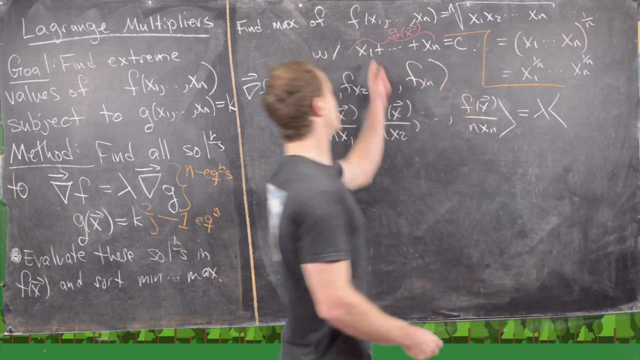 Then by the method of Lagrange multipliers. We need that to be equal to lambda times the gradient of g. so that needs to be equal to lambda. But notice, the gradient of g is super simple. the derivative with respect to x1 is 1. the derivative 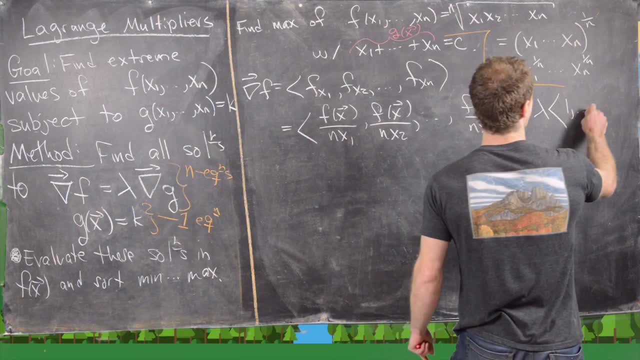 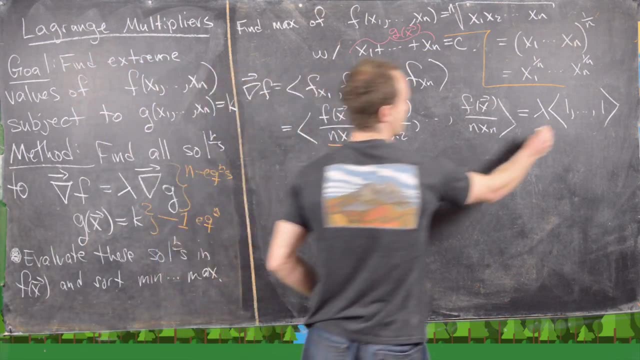 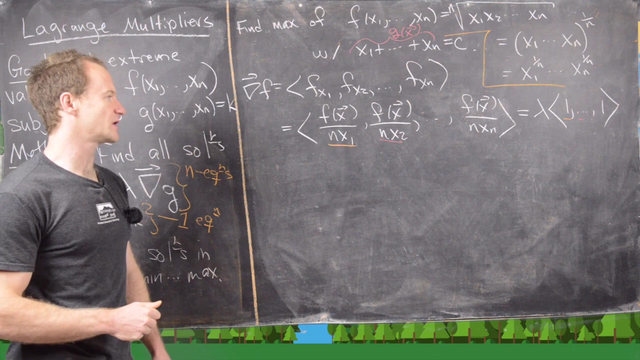 With respect to x2 is 1 and so on and so forth. so all of these are just 1. so now notice, we can take these and create n plus 1 equations and n plus 1 unknowns. so our n plus 1 unknowns are x1 to xn and lambda. 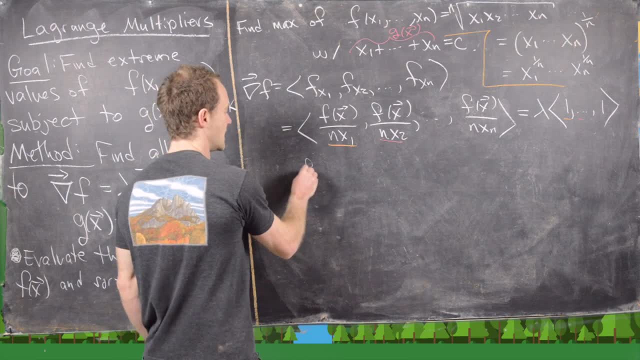 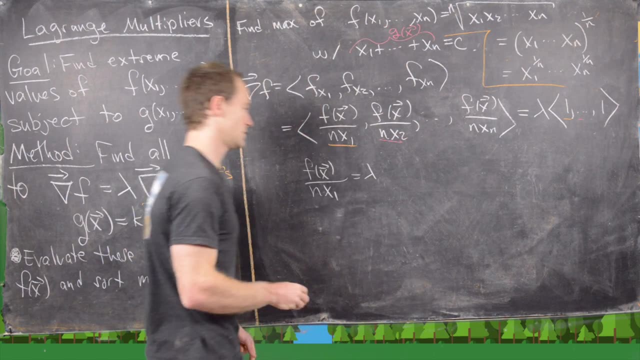 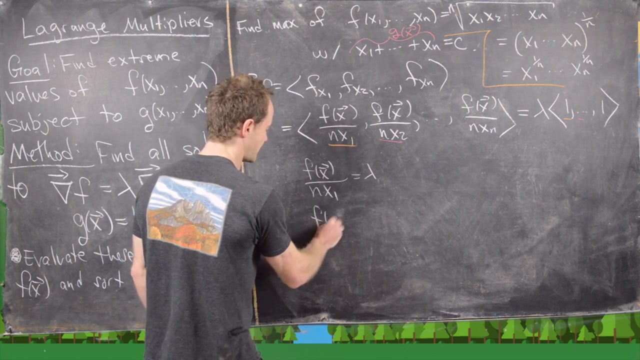 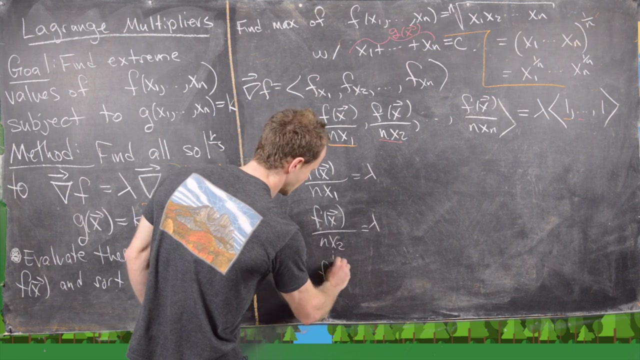 So our n plus 1 equations are going to be given by: f of x over nx1, equals lambda times 1, But then, so that's these orange underlines. but then the red underlines will give us f vector over nx2 equals lambda, and so on and so forth. so f x vector over nxn is: 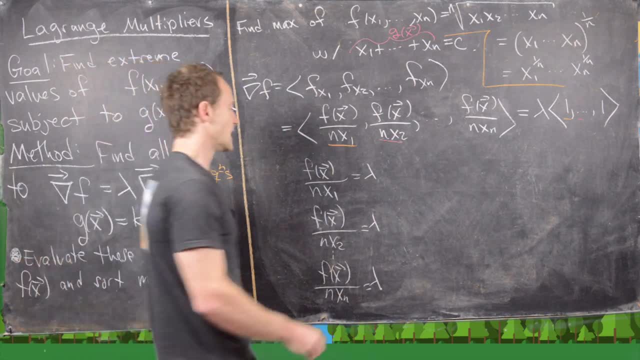 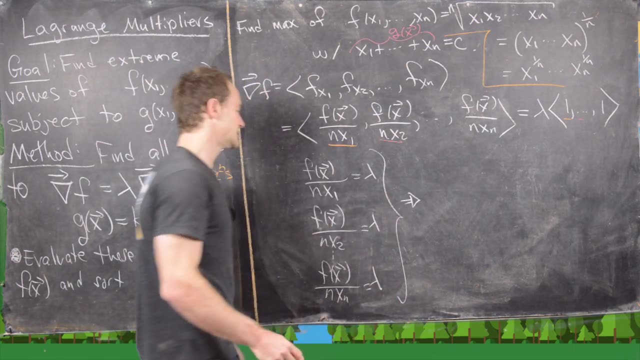 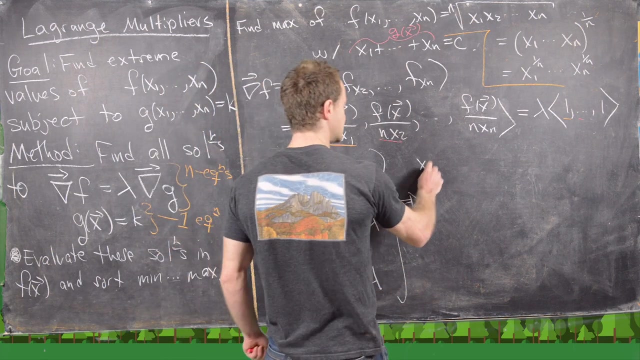 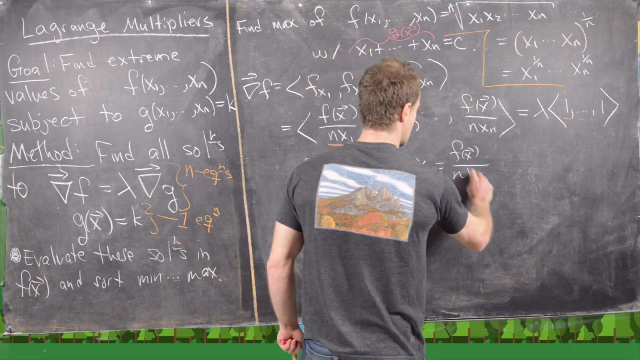 also equal to lambda, Okay, good. and then Notice all of those are the same. so what that tells us is that we can solve all of these for X, n and notice that this means that x1 equals our function divided by n times lambda, but then x2 also equals our function divided by n times lambda, and 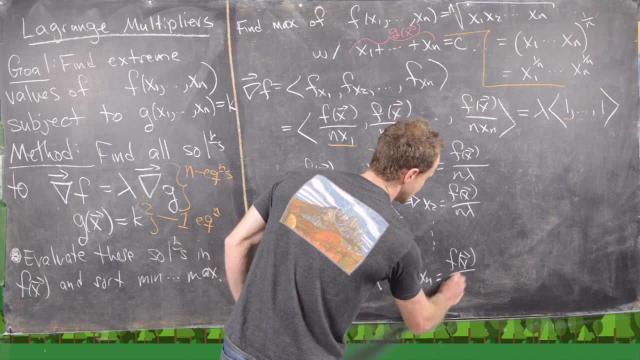 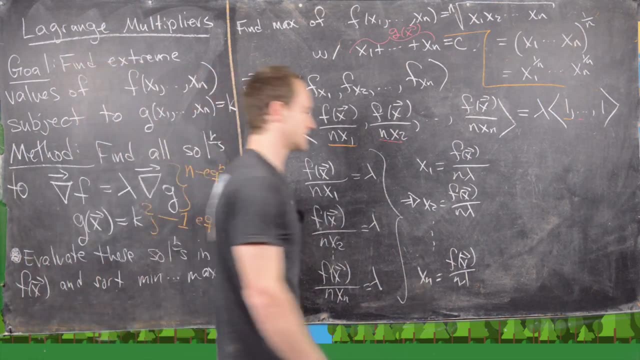 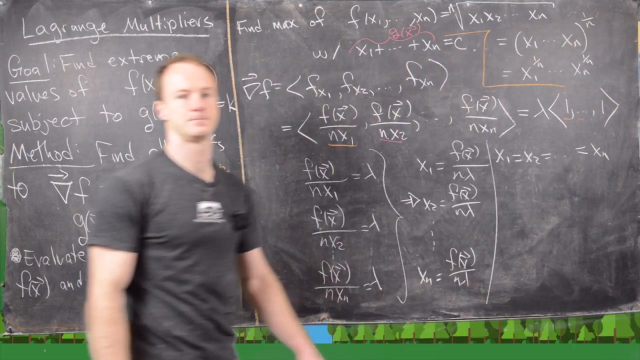 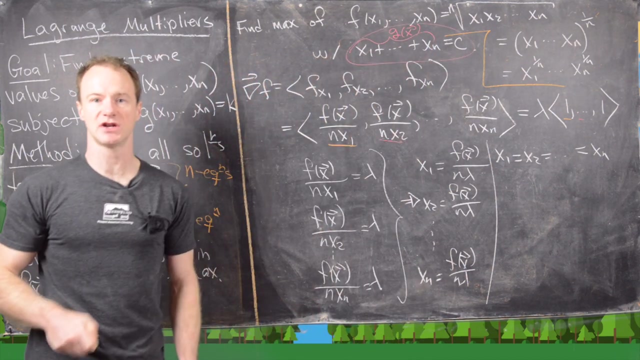 Xn is also our function, divided by n times lambda. so notice, every value of x is equal to the same. so notice we have x1 equals x2, All the way that equals xn. Okay, great, but now we can also use our Constraint equation, which is x1 up to xn equals c, and that will give us also we have 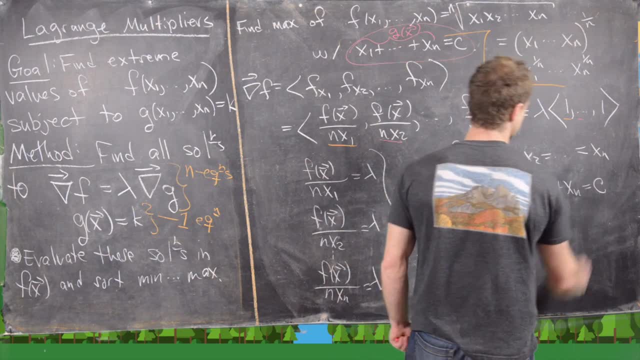 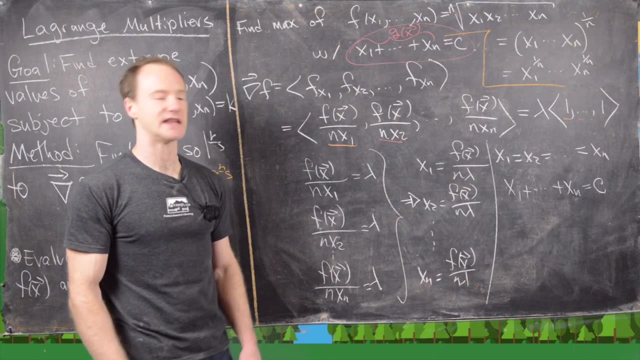 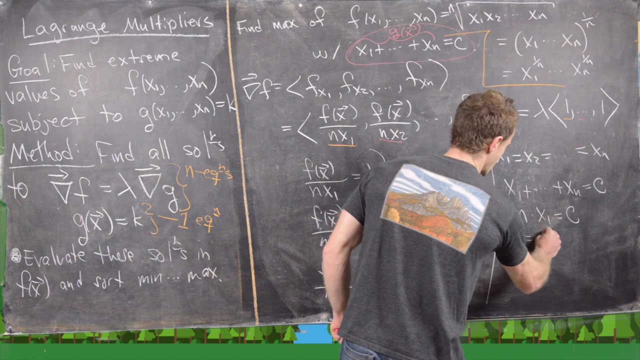 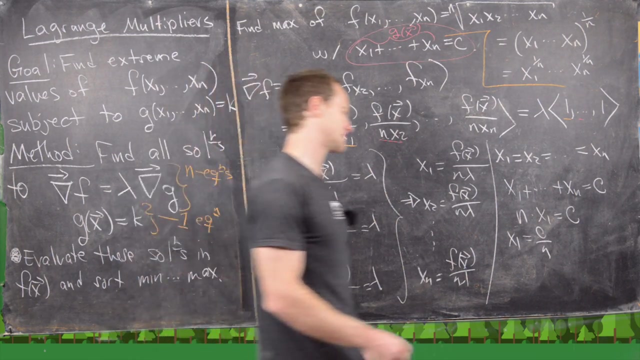 x1 plus up to xn equals c, But now we're adding a bunch of numbers. all of them are the same and we're getting c. So this is the same thing as n times x1 equals c. in other words, x1 equals c over n, But since x2 is the same as x1 and x3 is the same as x1, that means what we really have is x1 equals x2. 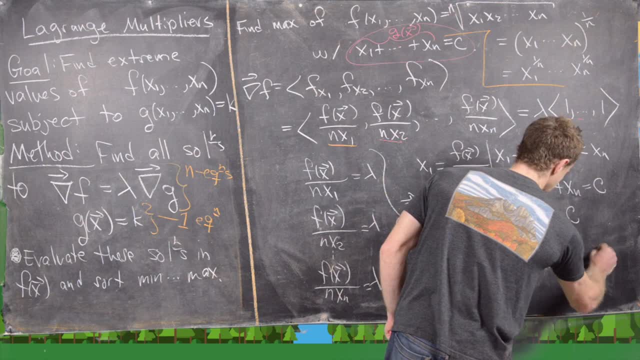 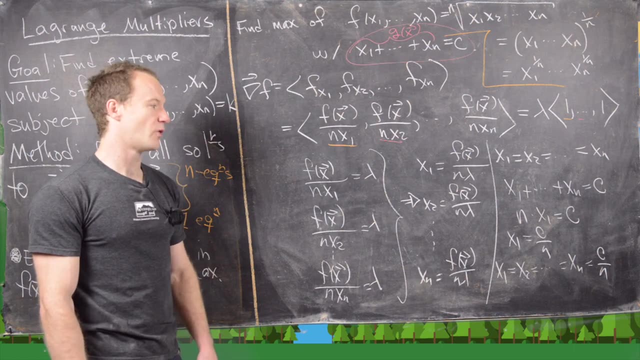 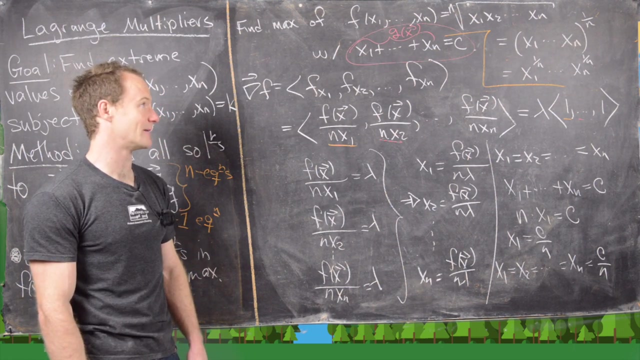 equals all the way up to xn. all of these things are c over n. Okay, good, So we found our point at which our maximum will occur. it will occur at the point where all of these values are the same. Now, the next thing that we want to do is find the maximum of this actual function. 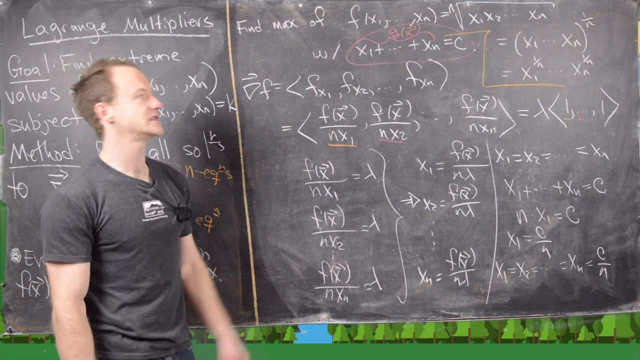 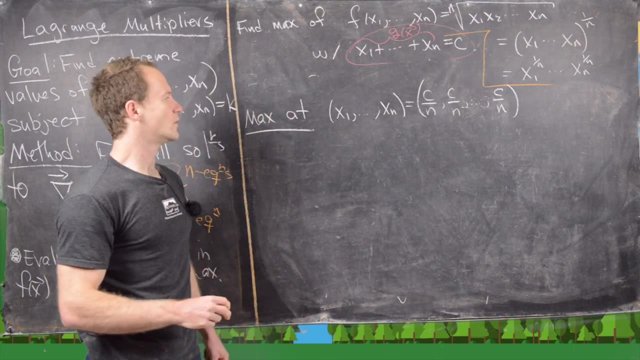 So we can do that by plugging this point into the original function. so I'll clean up the board and then we'll do that. Okay, so in the previous boards we had decided that the max is going to occur at this point: x1 to xn, where all of those are the same and they're 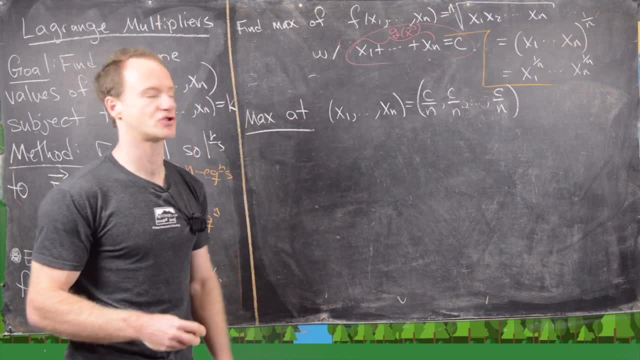 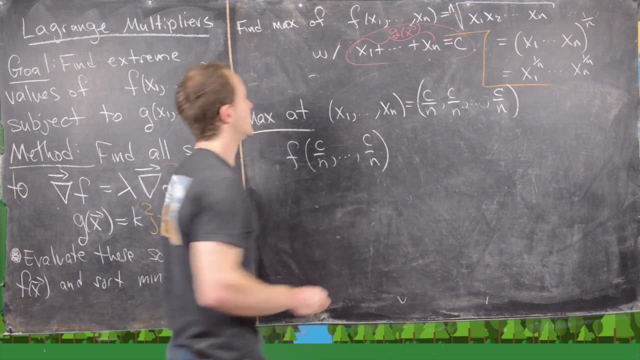 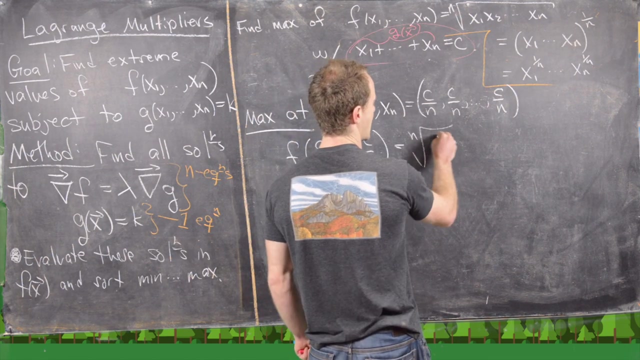 Equal to c over n, which we get by our constraint function. So now, if we go ahead and plug this into The function which is the nth root of this product, so we're going to get the nth root of This product, c over n, all the way up to c over n. 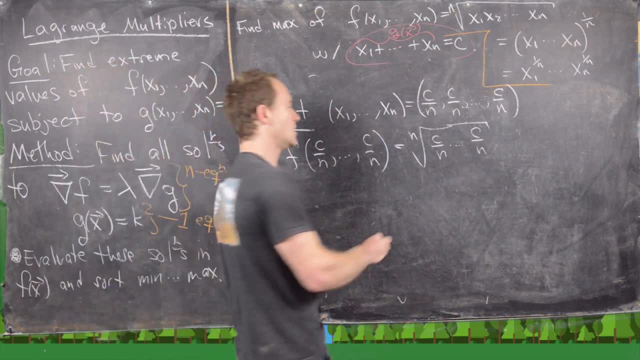 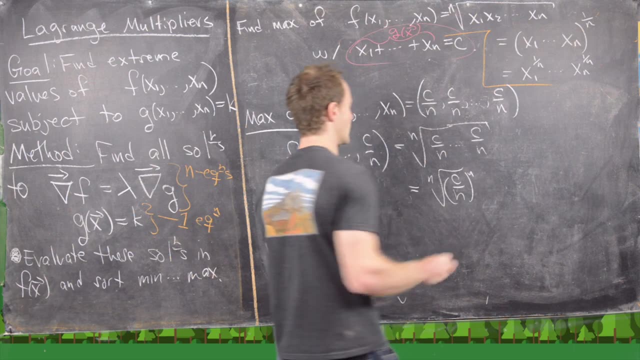 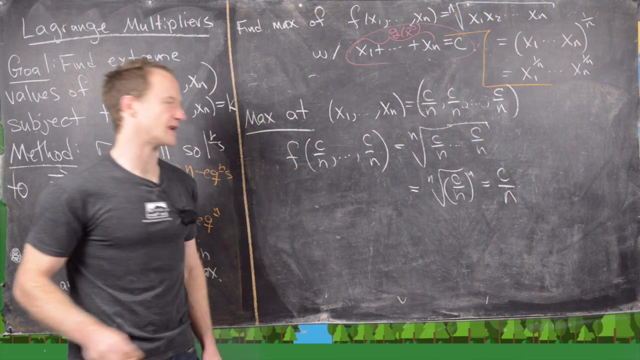 Okay, good, but now notice That's equal to the nth root of c over n, to the n power. Great. but notice that those are going to exactly cancel each other out and we'll get c over n. But now let's notice that c was equal to, via the constraint equation: 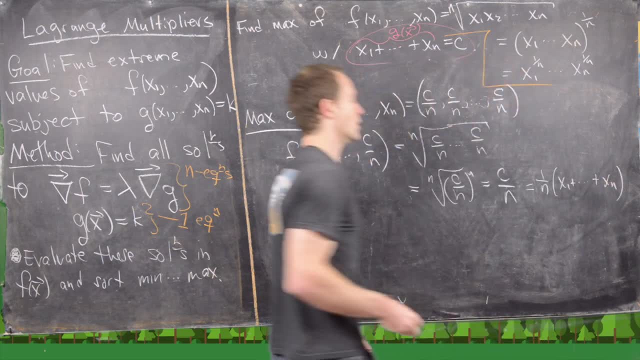 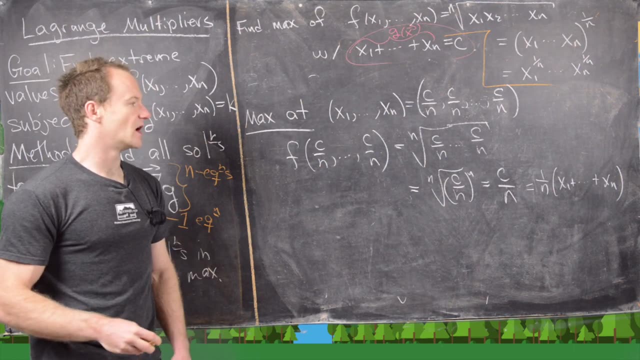 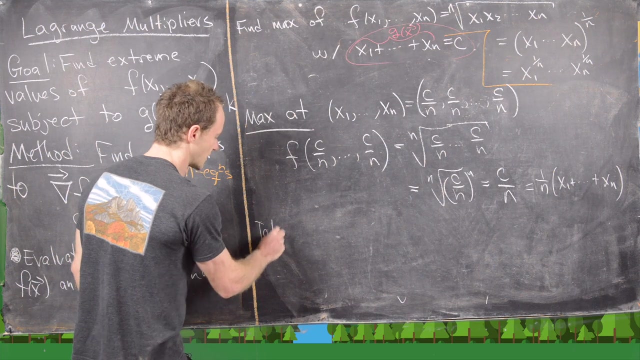 x1 plus up to xn. so what we really have is that This is equal to 1 over n times x1 up to xn, where obviously We've taken each of those x i's to be c over n. so anyway, the takeaway here Is: Since this is the maximum of this type of function,